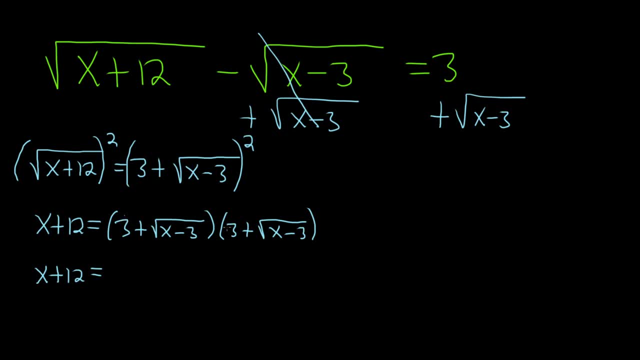 I just don't think of it as FOIL. We're just taking the 3 and multiplying it by both of these, and then taking the square root and multiplying it by both of these. That's the same thing. If you think about FOIL, it's first. so 3 times 3 is 9.. 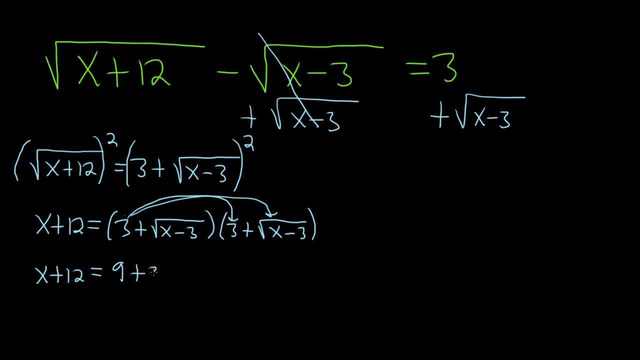 Outside so, or outer so, 3 square root x minus 3.. But basically what we did is we just took the 3 and multiplied it by both. Then we do the same thing with this one Boom This times this. 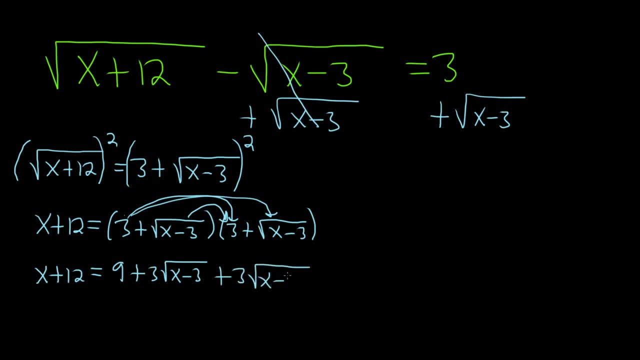 So 3 square root x minus 3.. And then this times this: So when you multiply these two, the square root will go away, because it's the square root of x minus 3 times the square root of x minus 3.. So the square will go away. So you just get x minus 3.. 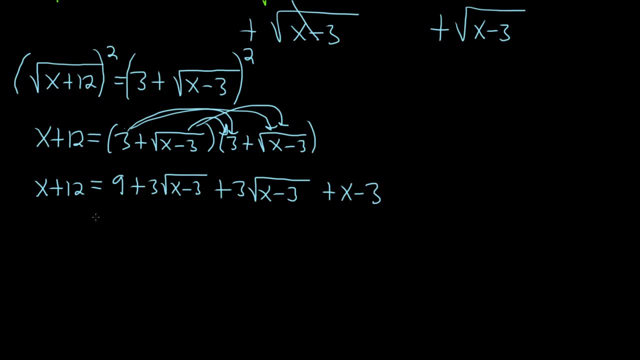 Alright, let's go ahead and clean stuff up. I think we have some like terms here on the right. So x plus 12 is equal to. let's see, The 9 and the minus 3 are going to give us a positive 6.. 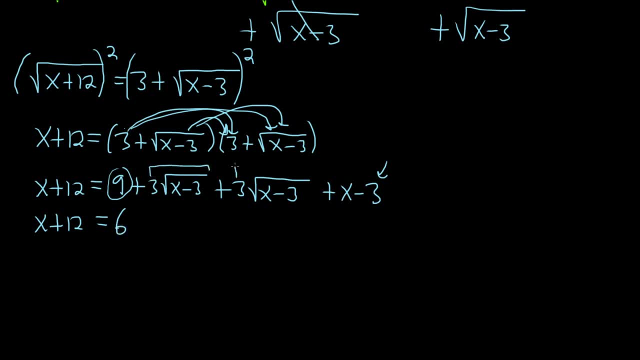 And then here in the middle we have 3 of these plus 3 of these. That means we're going to have 6 of those right. 3 plus 3 is 6.. And then we still have the x over here. so plus x. 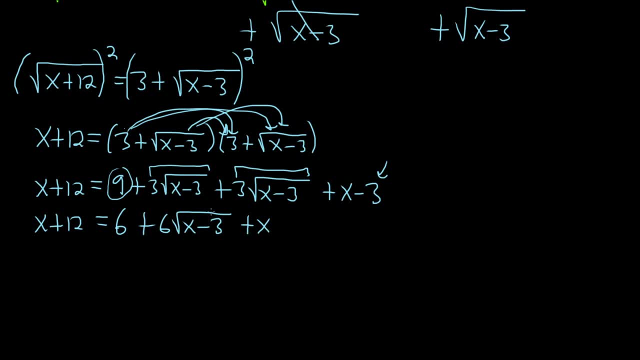 So we still have a square root. So we want to solve for this square root so that we can square both sides. So let's go ahead and isolate it And we'll subtract 6 from both sides. Boom. And let's go ahead and subtract x at the same time. 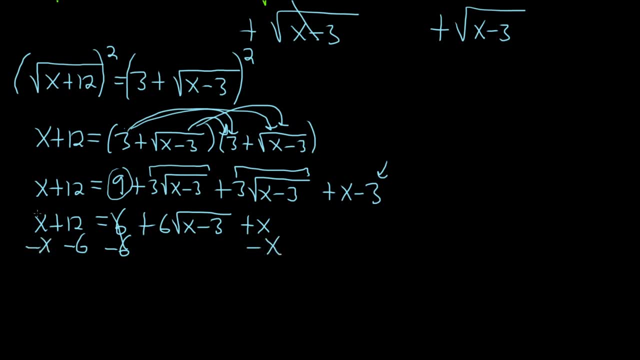 So minus x, minus x, Boom. So 12 minus 6 is 6. And that's equal to these. cancel as well 6.. Oh, this is nice. This is not so bad. It could have been worse. 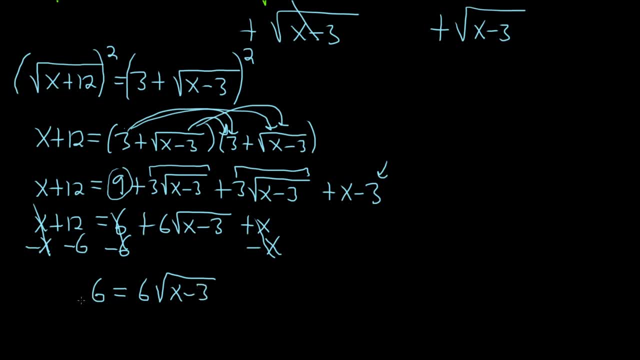 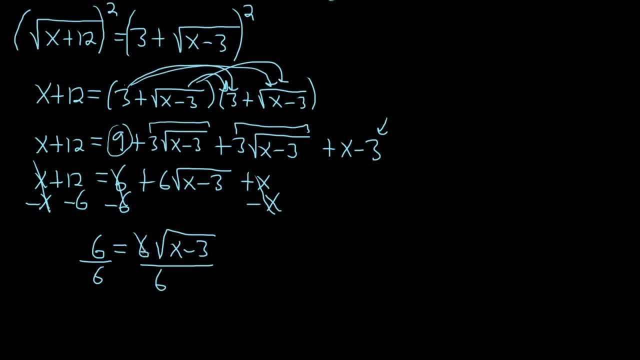 You know, we could have had like more x's over here. I was like, no, This is a nice one, Not super bad. And then divide by 6.. Divide by 6. So we get: 1 equals the square root of x minus 3.. 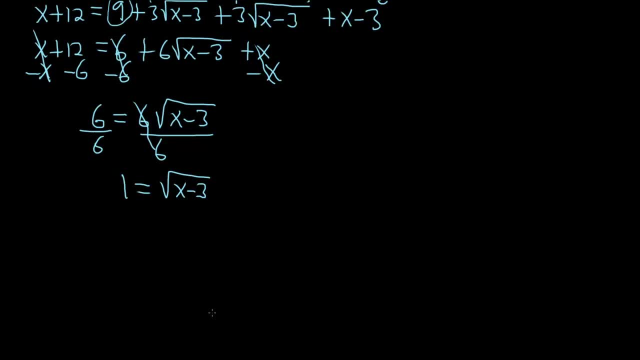 Good stuff. So now we need to get rid of the square root. So what do we do? We square both sides. Beautiful stuff. 1 squared is 1.. And on the right-hand side we get x minus the number 3.. 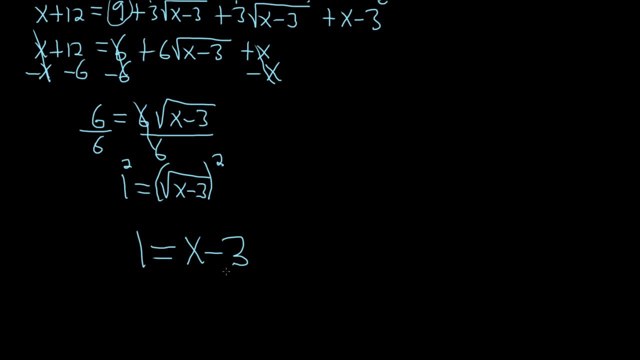 We're almost done. I'd be really bad to mess up here. All we have to do is add 3 to both sides, So plus 3, plus 3.. And so you get x equals 4.. Now, is that the answer? 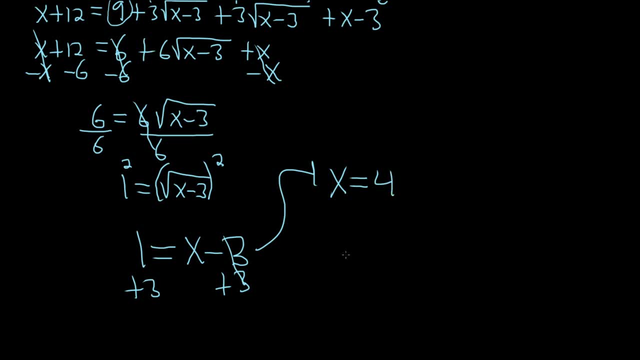 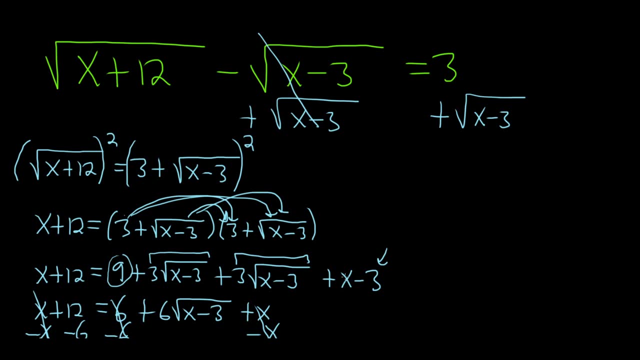 Well, the honest answer is: I don't know. We have to check. So whenever you have equations with square roots, it's super important to check. So I'm going to write down the original one: x plus 12, x minus 3.. 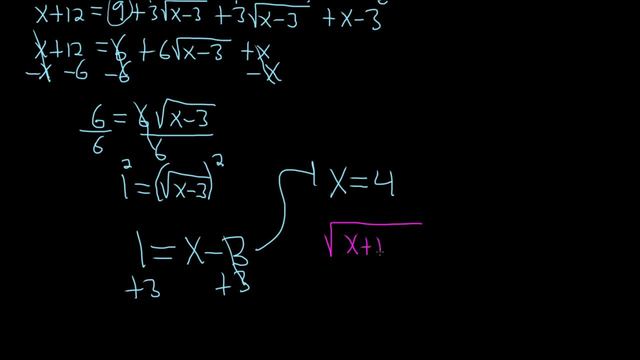 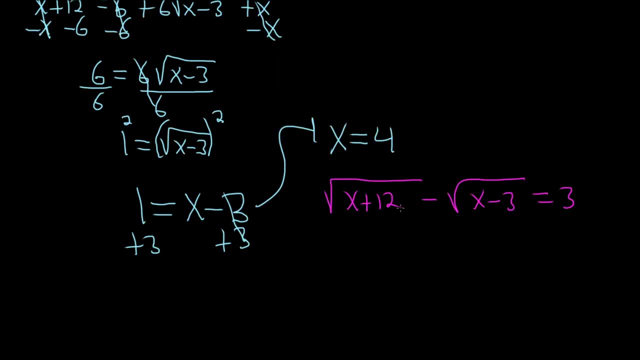 Let's see, So it was. this is the original question. x plus 12 minus the square root of x minus 3 equals 3.. And so when you check, it's important to you know, it's important to take your value of x and plug it into the original. 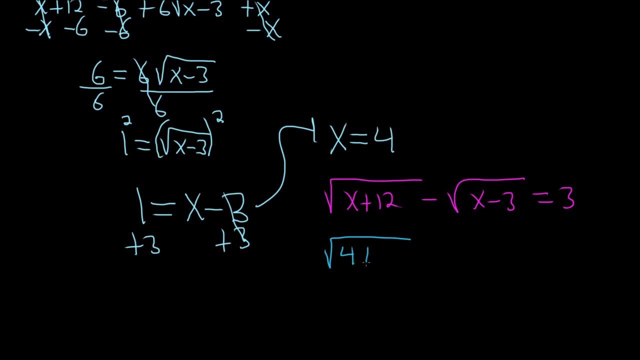 So let's do that. So we have the square root of 4 plus 12.. So we're checking for minus the square root of 4 minus 3. And that might be equal to 3. We'll find out, So let's see. 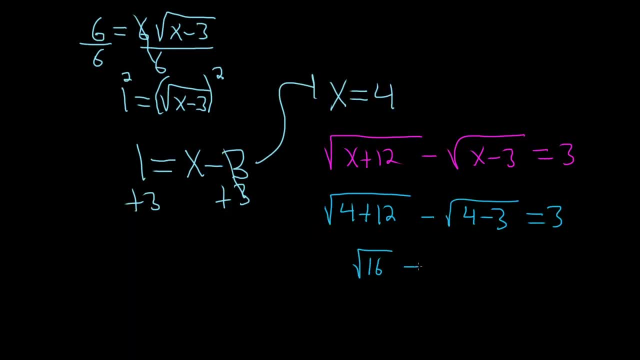 4 plus 12 is 16.. So we have the square root of 16 minus 4 minus 3 is 1.. So square root of 1. And that should be equal to 3, maybe. So 4, right. 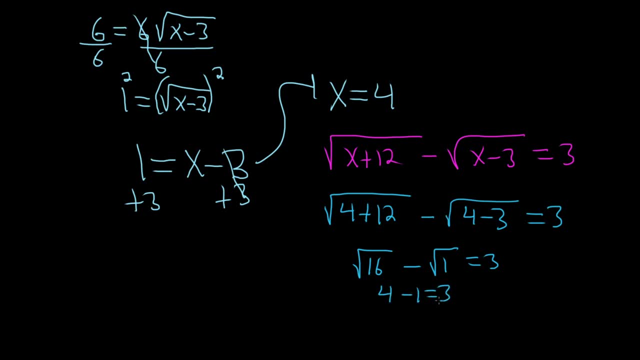 Square root of 16 is 4.. Square root of 1 is 1.. So 4 minus 1 is 3.. So 3 is equal to 3.. Yes, it checks. So that is the answer. So this is the answer. 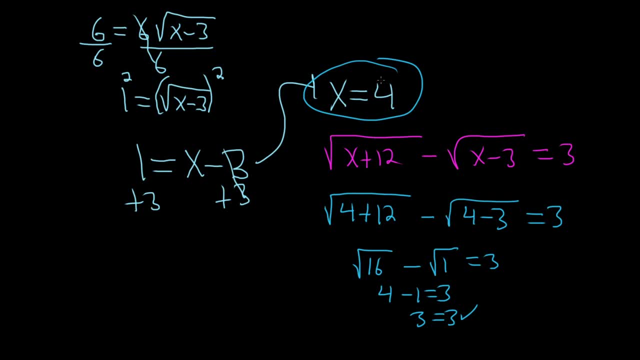 If it wouldn't have checked, then in this case there would have been no solutions. That can happen. It's really important that whenever you have square roots, always, always, always check your answers at the end. I hope this video has been helpful. Good luck. 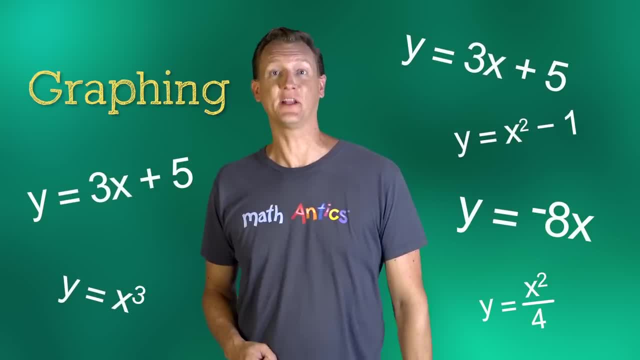 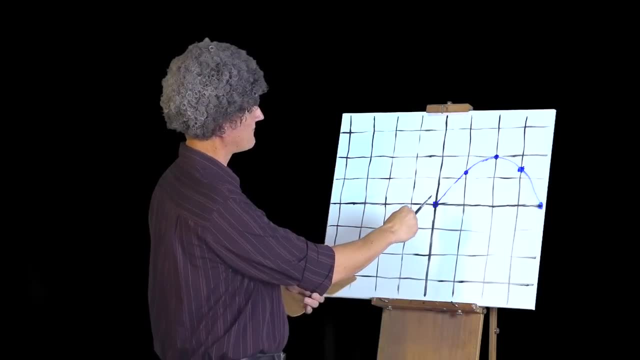 basically means taking mathematical relationships and turning them into pictures. Hey friends, welcome back to the Joy of Graphing. We're going to pick up right where we left off. We already have this nice, beautiful function right here, but it needs a friend. 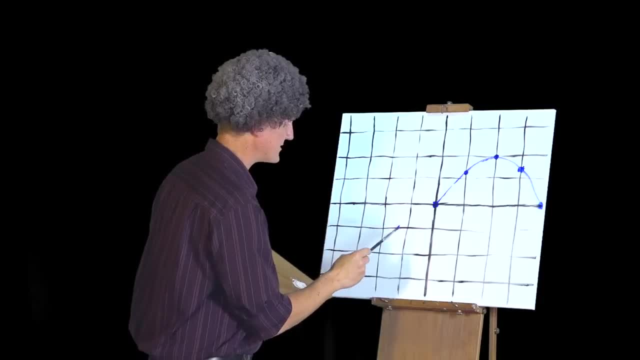 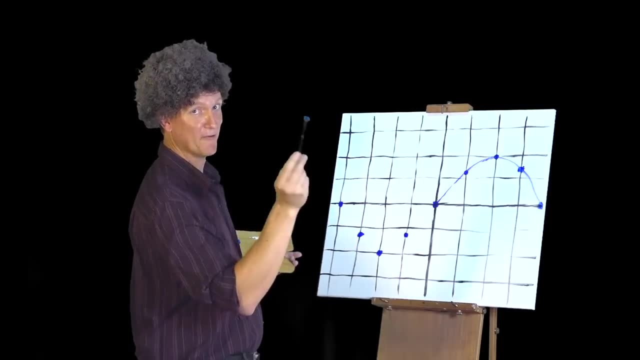 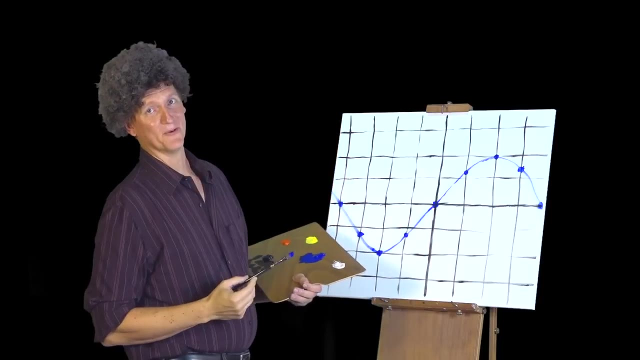 And we're going to do that by adding some points. So let's put the next point right here. Now, all we need to do is connect those points, Because they're all friends. And what do friends do? They stay connected. Oh, and look at that, That's beautiful.